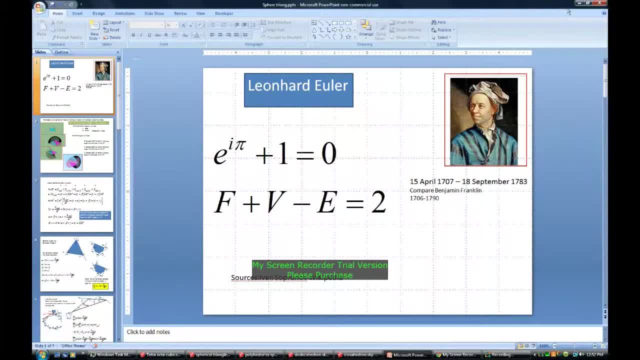 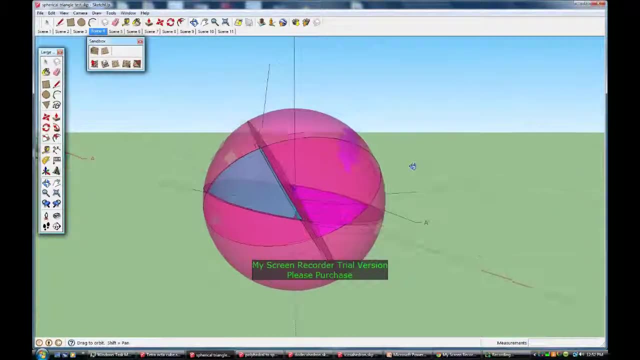 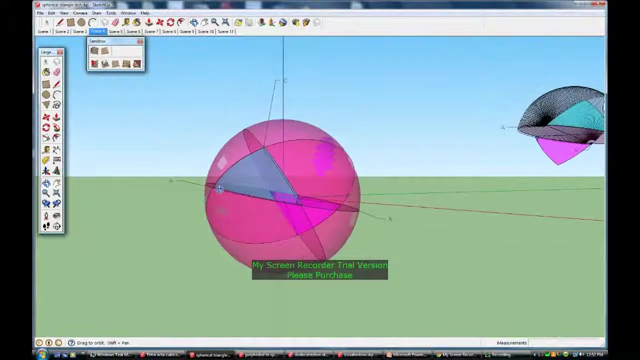 He lived approximately the same lifespan as Benjamin Franklin. He would have been dying shortly after the American Revolution started. Okay, So a spherical triangle is just a triangle on the surface of a sphere instead of being on a plane. So if you take a look at this thing here, 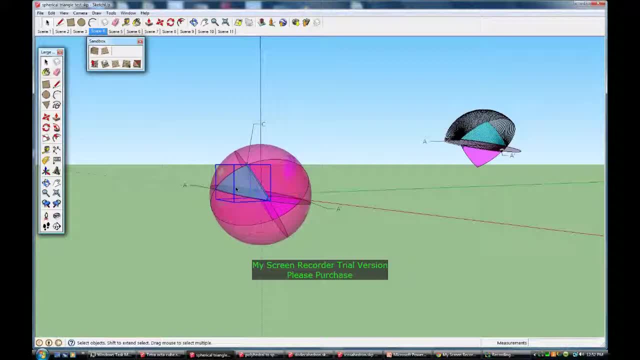 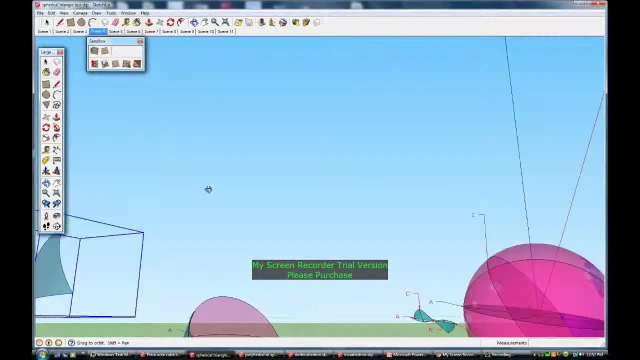 let's just highlight that and pull off just the triangle, which is something we can do with SketchUp, that you really can't do otherwise. So you see, you have this kind of curved surface instead of a flat surface, And that has consequences for the geometry. 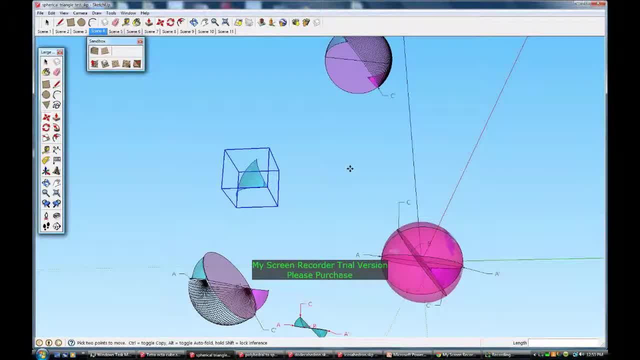 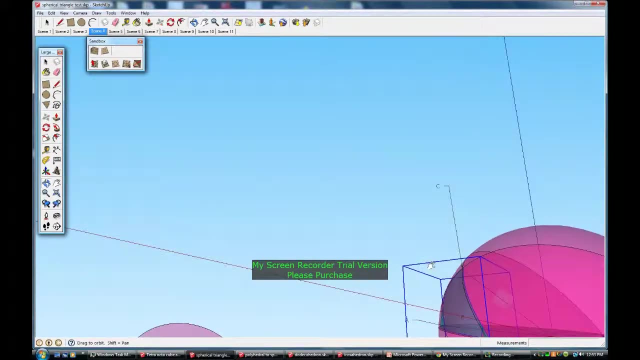 But there's things you can do with spherical trigonometry that you couldn't otherwise do, So I'll send that back and come in here, And I think SketchUp is a good tool, at least potentially, for studying these kinds of things. 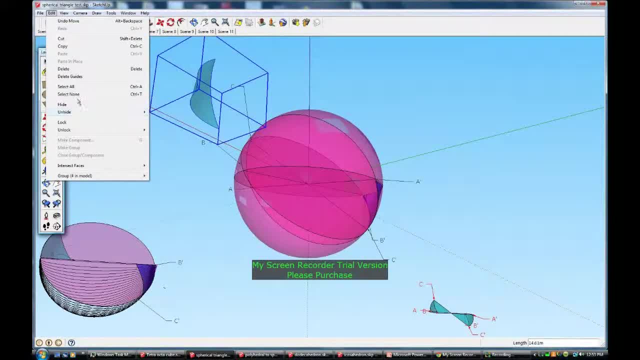 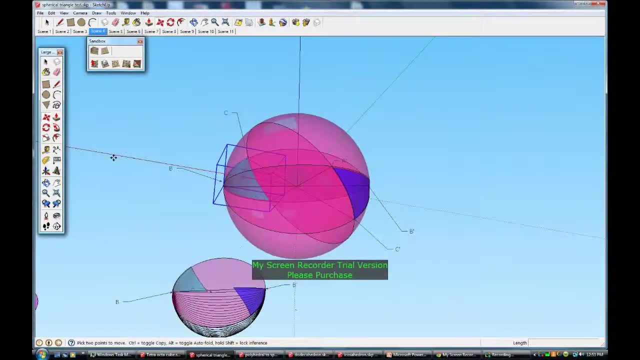 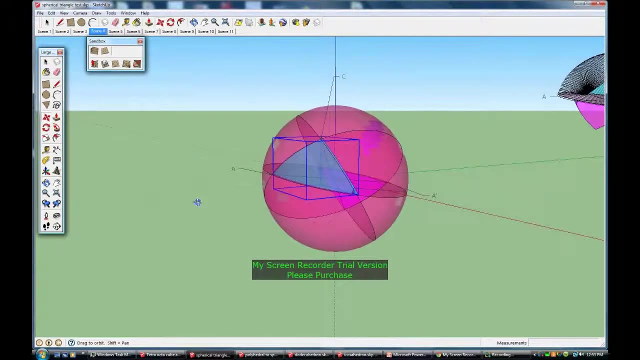 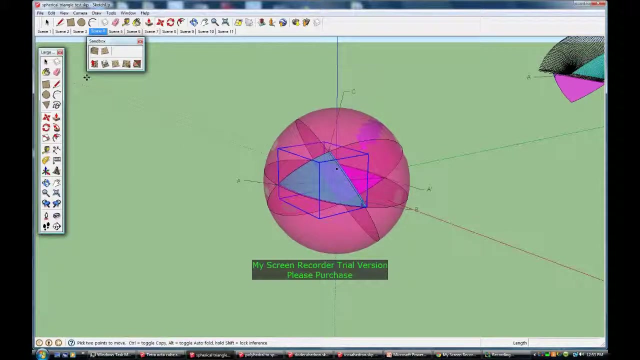 Let's kind of undo that. So you basically have three points here on the surface: A, B and C- But they're not connected by just straight lines. They're connected by what's called great circles, Circles that are centered at the center of the sphere and run along the surface. 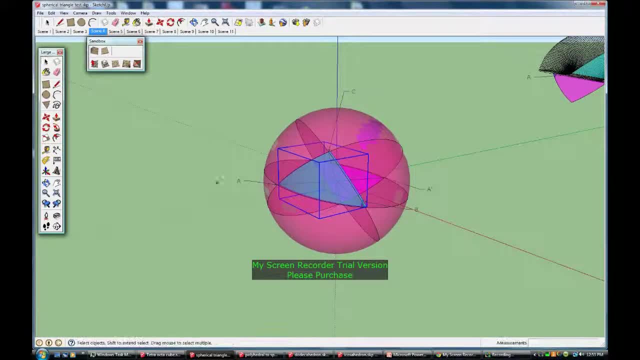 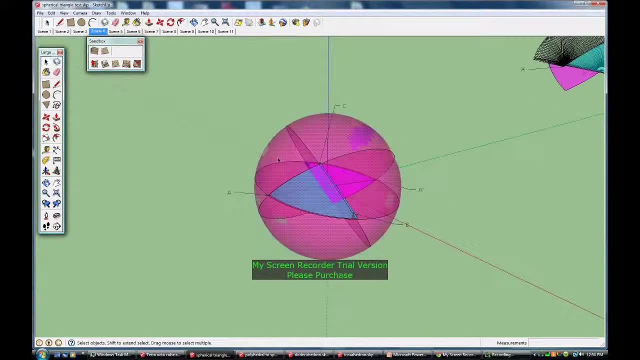 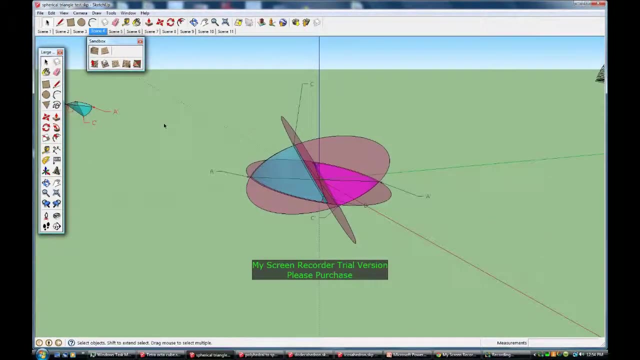 So that's really the largest circle that you can have on the surface of a sphere, If you just take these, if you take the sphere off. Let me just hide that for a second. See what it is. The straight lines between A and B and A and C are replaced by these arcs. 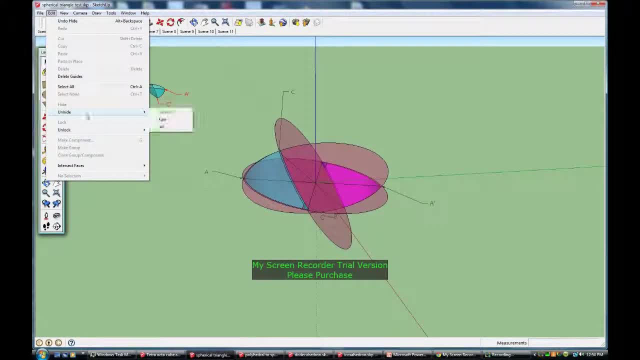 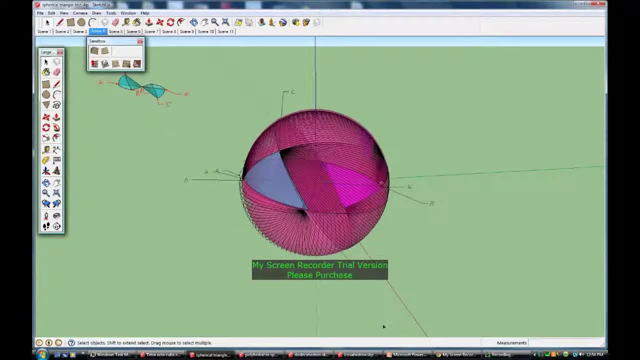 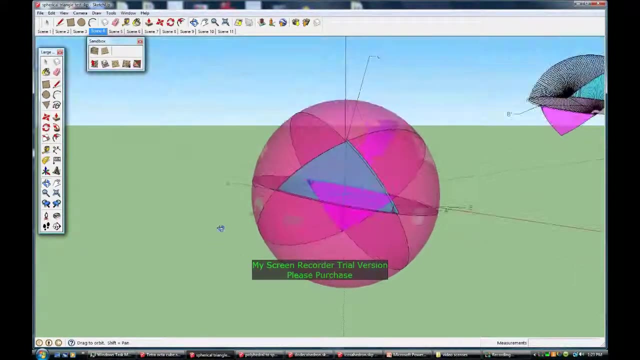 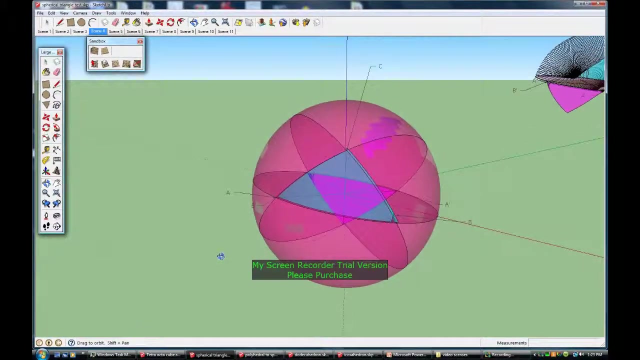 So that's the principal difference. All right, So if you accept the idea that there can be triangles on spheres just like there can be on flat space, connected by arcs rather than straight lines, and the arcs are parts of great circles, which are circles centered at the origin and having the same radius as the sphere itself, 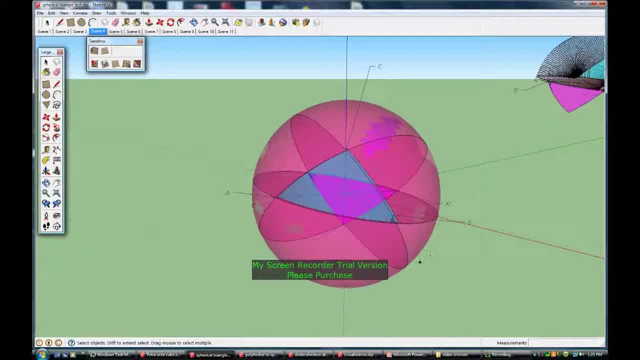 So you have this one- A, B, C- And the first thing you get when you put a triangle on a sphere, or one of the first things you might notice is you get another triangle on the opposite side. So this triangle is a little bit transparent. 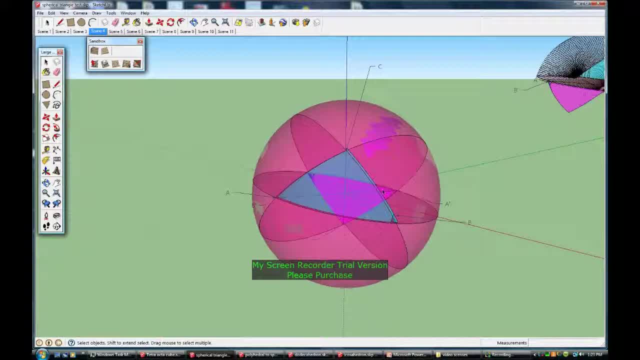 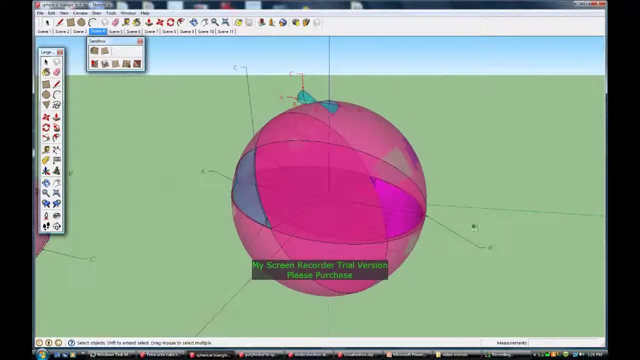 So you can see there's another triangular shape that's sort of an upside down version And what that is. you take the point A, the first vertex, draw a line to the center of the sphere and out to the back surface of the sphere to get to this point, A prime. 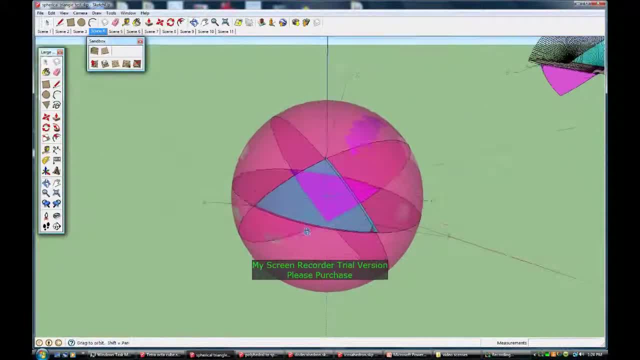 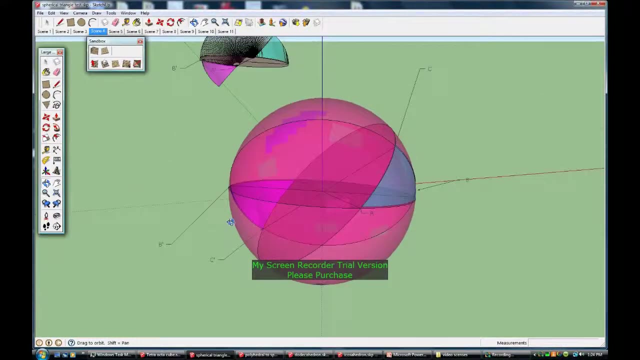 And that's the vertex of the inversion triangle. And then you come here to B, The B vertex of the triangle. Do the same thing and you'll come to B prime, The B prime index, the vertex of the other inversion triangle. And the same thing with C. 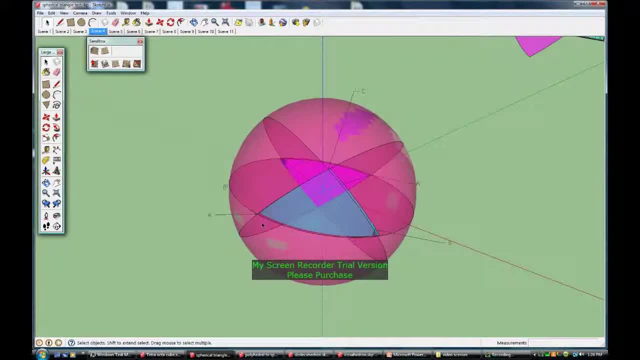 So you end up with a triangle on each side And you can pull that off. since you're working in SketchUp, you can pull that off, just that little, those pair of triangles, and look at them in isolation. Let's just do that, Alright. 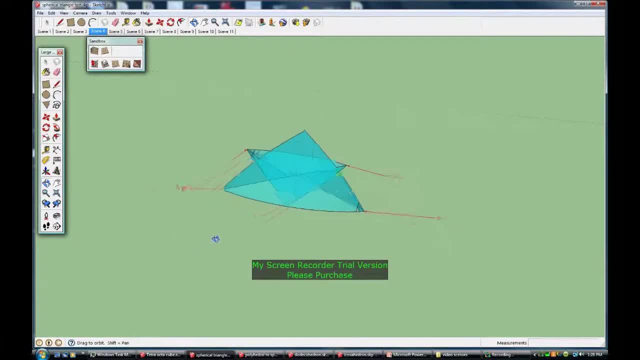 Now here are the two triangles just pulled off in isolation in SketchUp And you can see them quite nicely: A, B and C. There's the spherical surface And here are the straight lines through the center of the sphere and coming out on opposite sides. 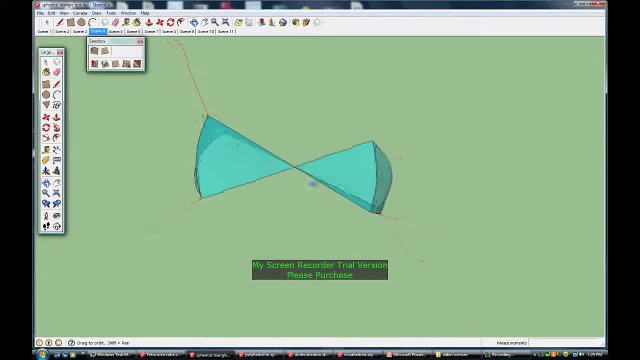 So there's C going to C prime, B going to B prime and A going to A prime, And you see, you just get two identical columns, Two copies, But that's an one, is the inversion through the center of the other, And that's just. 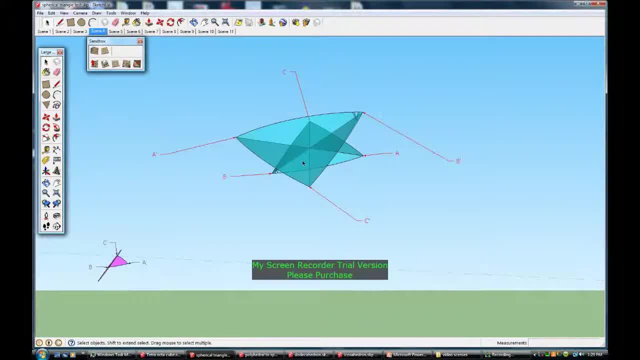 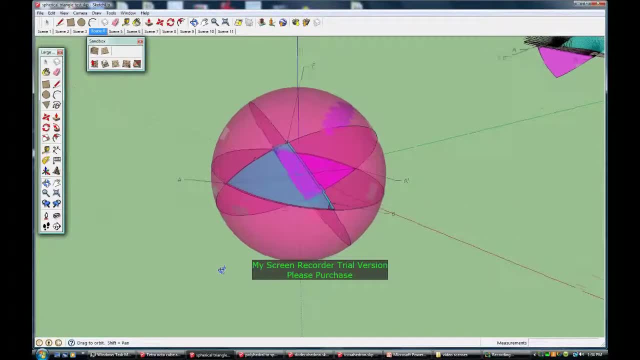 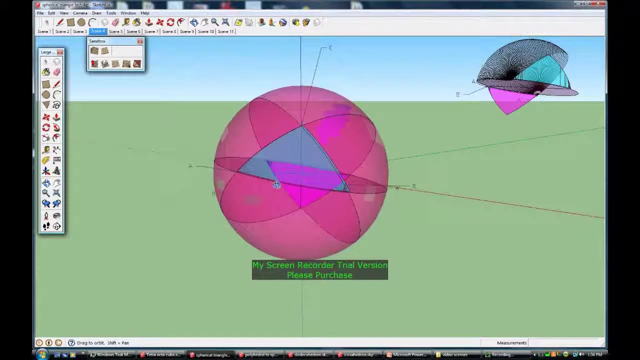 you know some one difference or one interesting aspect of spherical triangles. Alright, Another difference that you get when you add a spherical triangle on the surface of a sphere is you get what we can call biangular polygons. You know, On a plane a triangle is. 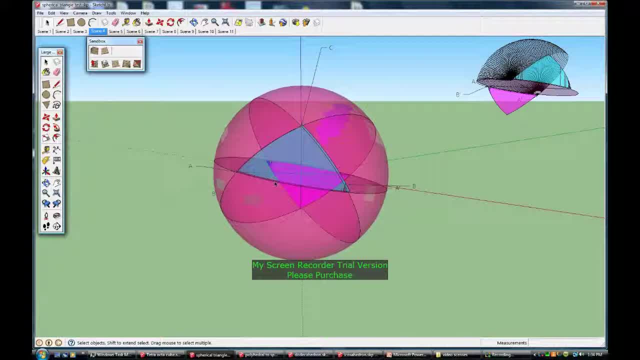 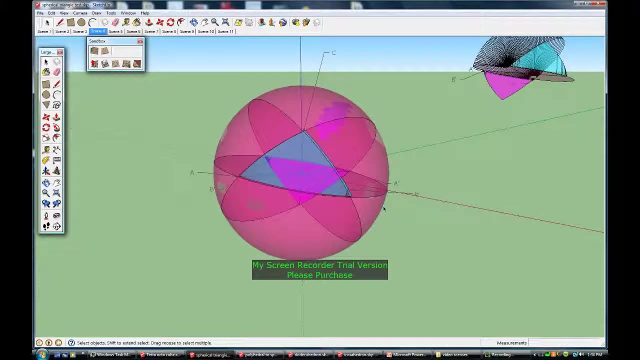 the simplest polygon you can get, You know a closed figure with straight line edges. But on a sphere you can get a biangular region And I'm going to show that. as soon as you draw a triangle, it's easy to generate three biangular regions. 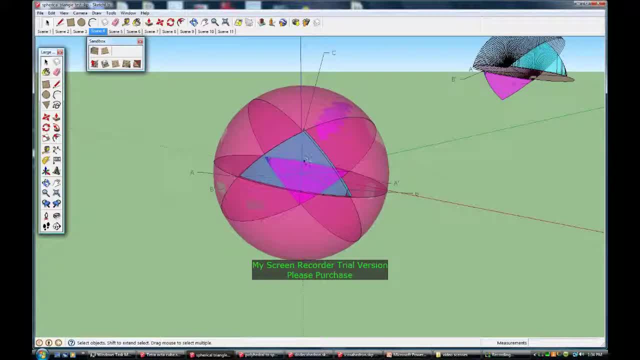 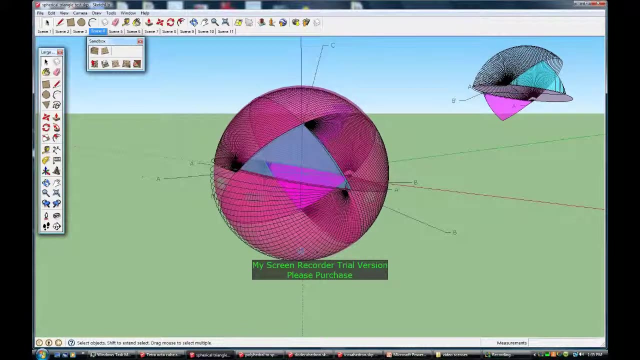 that cover up the remainder of the sphere that's not covered up by the triangle and its inversion triangle. So let me just show. there they are, the biangular regions. I just added them. I drew them with these kind of nets here, But what you have is like: 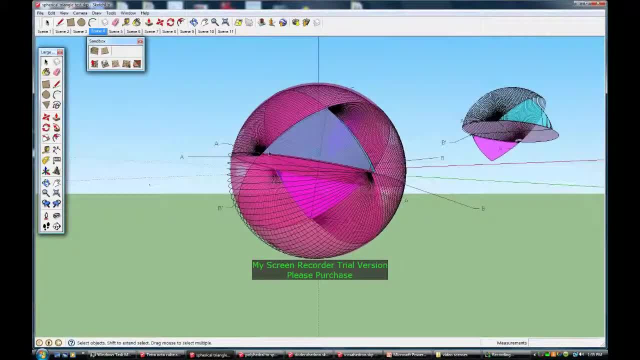 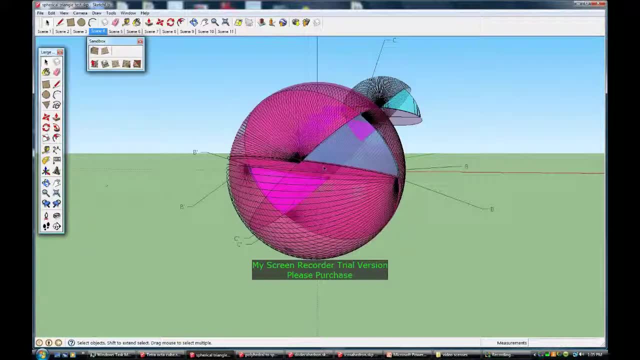 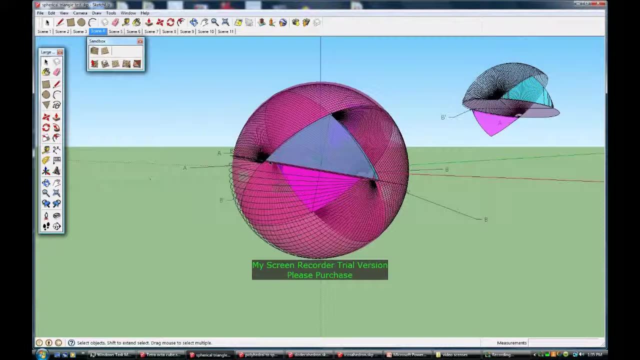 you have the triangle, let's say at point A, at vertex A, and then you have a biangular region. the angle of the biangle is the complement of the angle A. And I have that and I'm going to show that each, how those are, those regions are constructed. 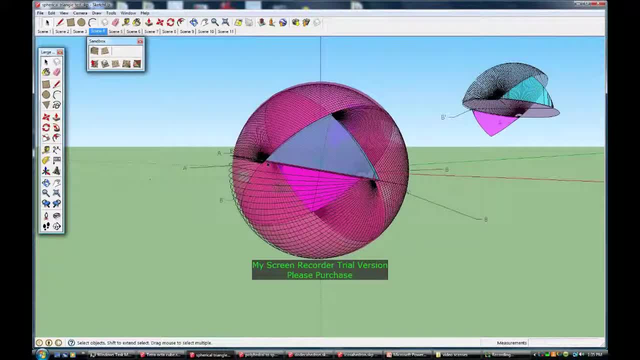 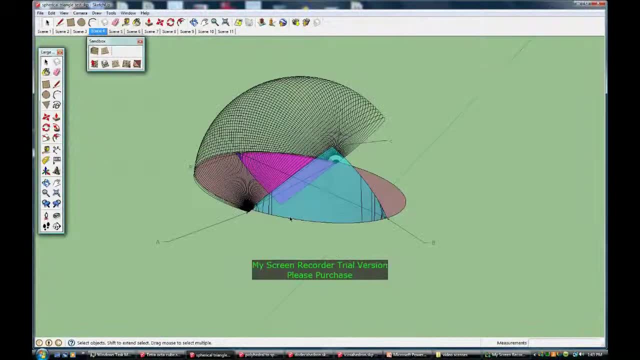 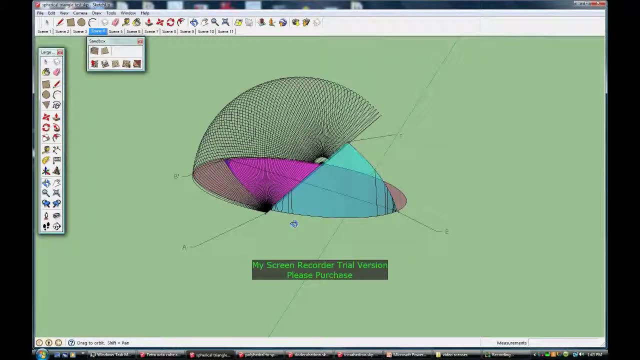 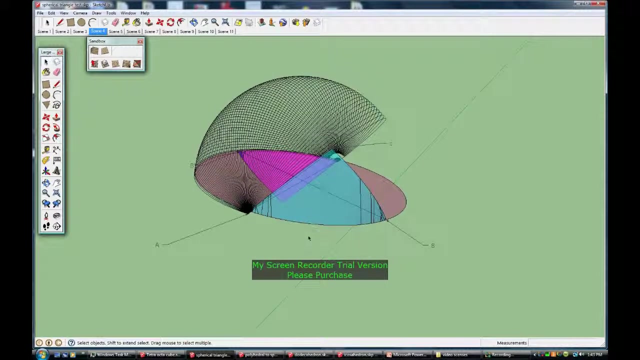 one at a time for each vertex of the spherical triangle. Alright, Now I want to show how you can construct a biangular surface at the, at the vertex A of a random triangle on the surface of a sphere. So I just isolated the triangle and the biangular. 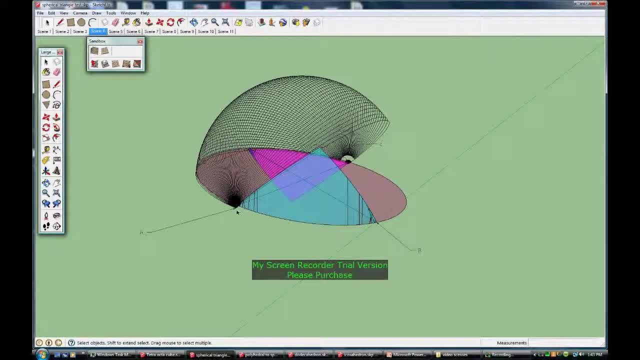 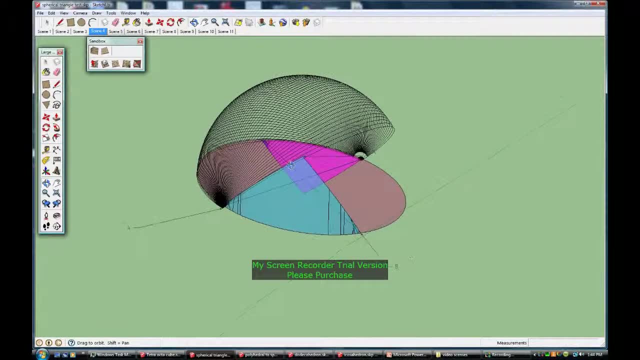 region that I want to illustrate The way you do this is: you start at the point A, you run a great circle up to C, just like you did to construct the triangle, but you keep going around until you get to A prime, But instead of continuing,